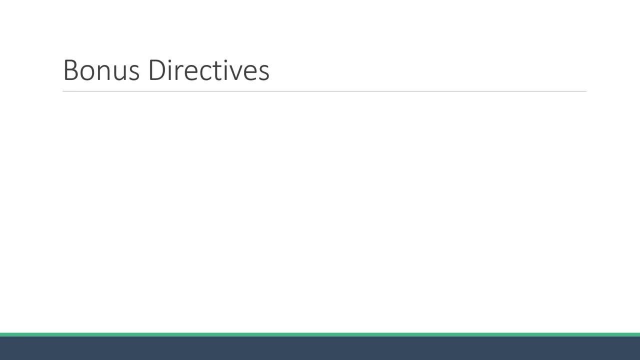 Alright, guys, in this video I want to quickly go over two more directives that Vue offers. They are the v-once and the v-pre directives. I can probably say that both these directives are less popular in terms of usage. However, I want to ensure that you are aware of their. 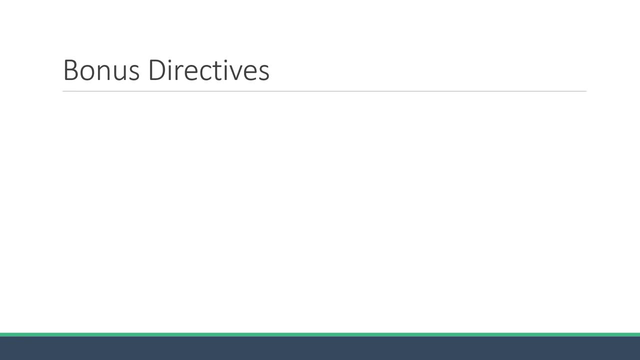 functionality in case you come across them in a project codebase in your company. Now, first we have the v-once directive. This directive, as the name indicates, renders the corresponding HTML element only once. On subsequent re-renders, the element is treated. 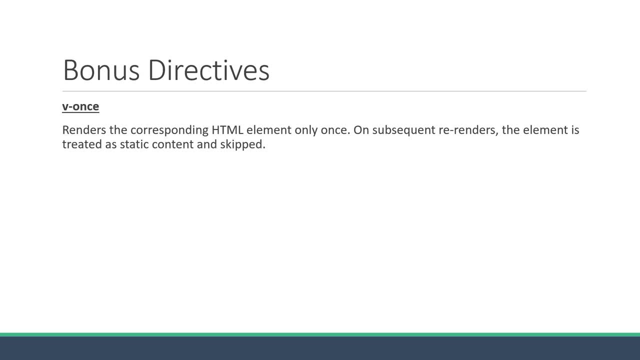 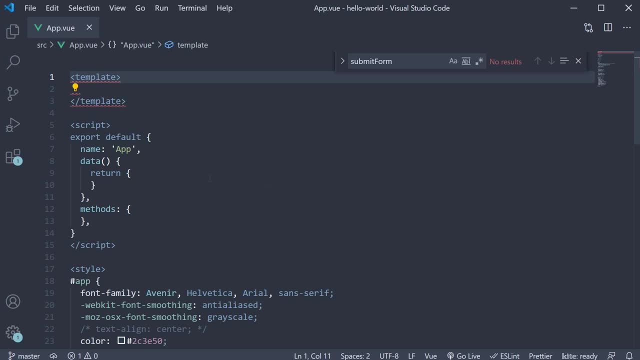 as static content and skipped. Let's understand with an example. We are starting fresh with an empty template and data object. I'm going to create a new data property called name and set it to v-once In the template. I'm going to bind this name property using the mustache syntax. 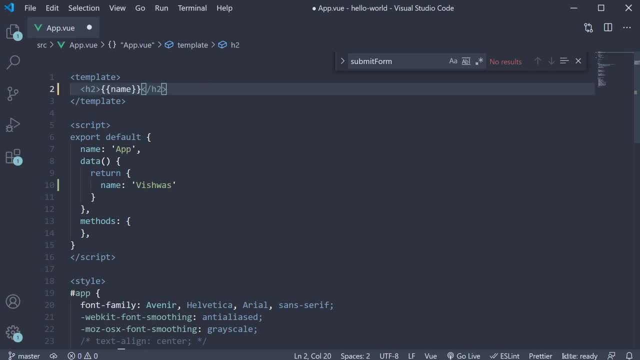 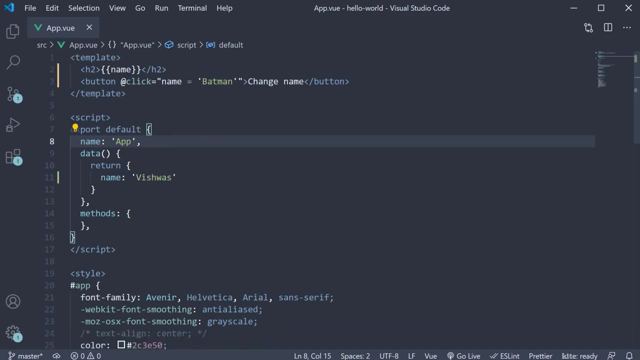 I'm also going to add a button to change the name. So button change name. On click we change name is equal to Batman. If we take a look at the browser, we have the name as Vishwas and on click of the button. 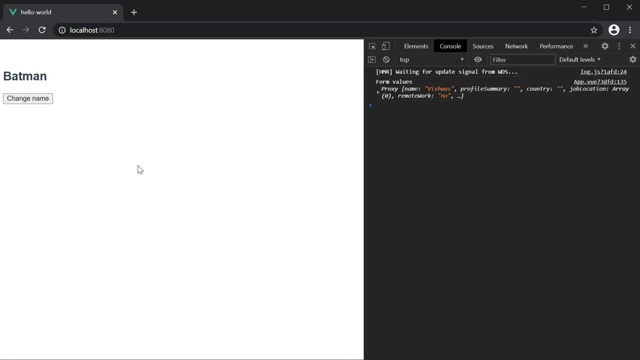 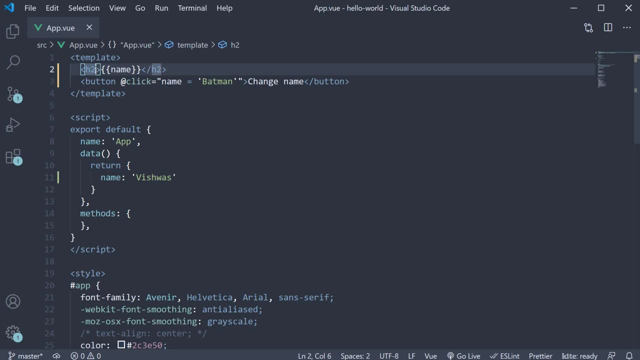 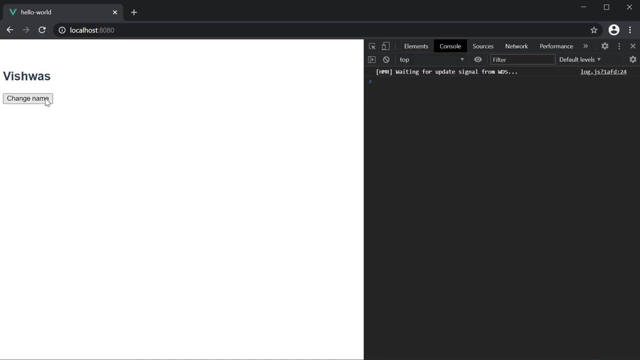 it changes to Batman. However, if we go back to VS Code, add the v-once directive on the h2 element and go back to the browser again, refresh and click on the button. you can see that the name does not change after it has been rendered once. 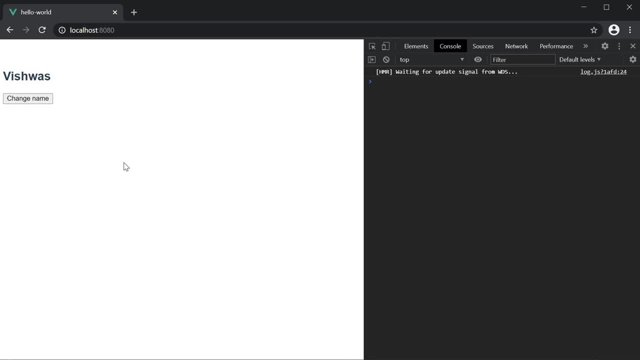 This directive can be used to optimize update performance. when used on a large portion of your template, This directive will skip diffing of the virtual DOM for the elements marked with v-once directive, thereby optimizing the update performance. It's pretty rare that you might come across very slow updates, which is why this is one.